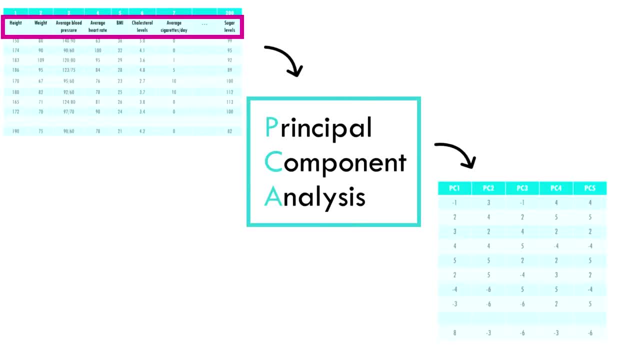 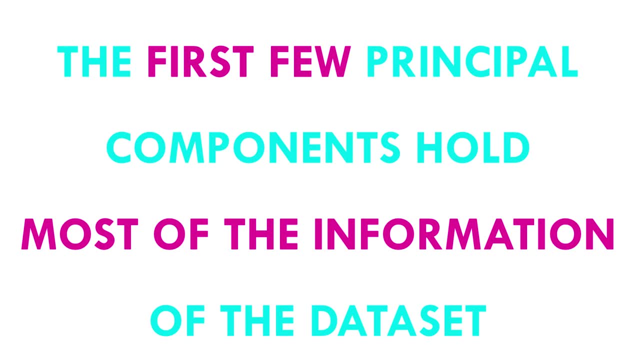 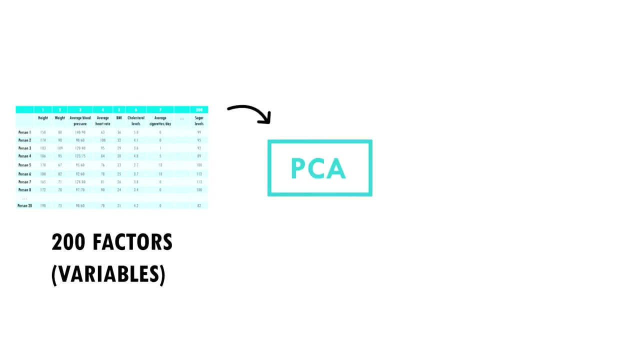 factors are called principal components, And it does that in such a way that if you focus on just the first few components, you will keep most of the information from the data set. Going back to our example, imagine we computed principal components analysis on our data set and reduced 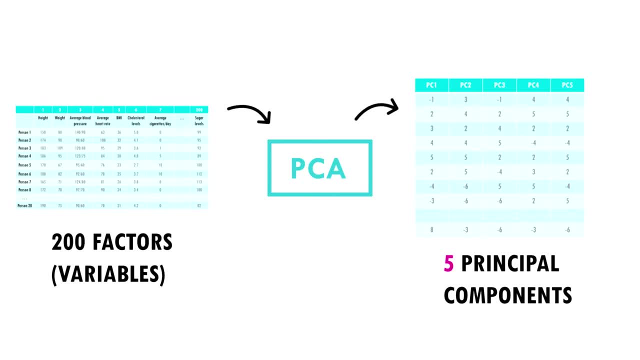 our 200 dimensions to five principal components. So we have a set of five principal components in our data set. This is amazing. We were able to simplify the data much more And, what's important, we didn't lose much information. Okay, but we cannot represent five dimensions in a 2D. 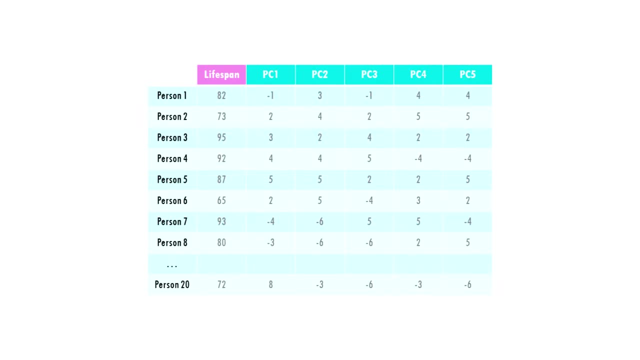 plot. The nice thing about PCA is that principal components are ranked from most important to least important. So let's just plot PC1 and PC2.. This is our PCA plot, And each point is a person from our data set. What if we colored the points by age? we can see that our samples already. 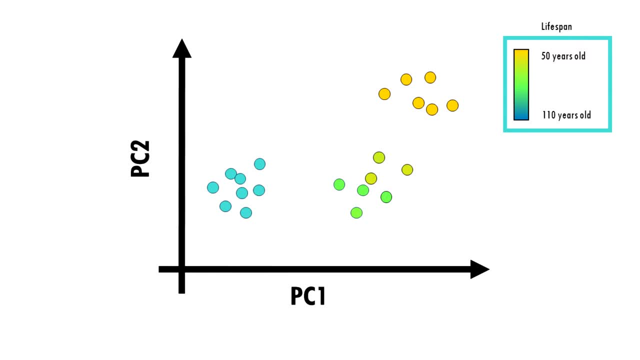 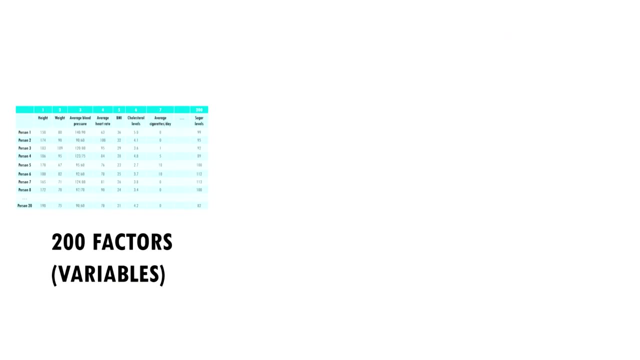 clustered together really nicely by age. Those people who live longer seem to be grouped together, those who live shorter tend to be grouped together. So PCA took into account all our biological factors, transform them into a new variables called principal components, And if we just take the first two we actually already see some interesting trends in our data. 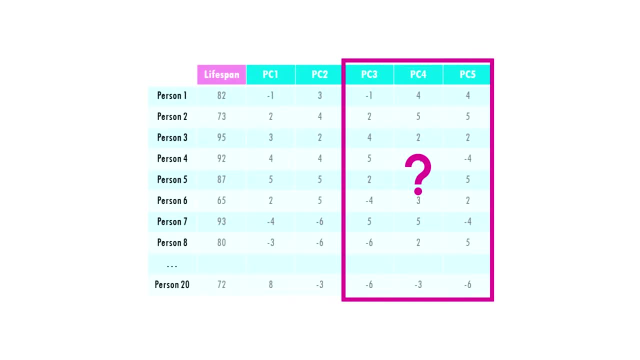 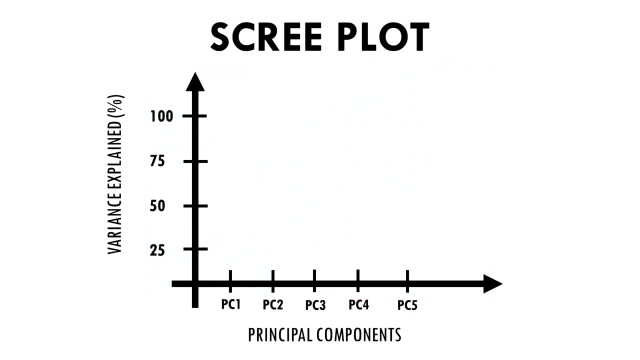 But what about the other PCs? How do we know if the first two principal components are enough to capture most of the information or variance in the data set? Well, the solution to this is a scree plot. A scree plot tells you how much variance of the data set, basically how much. 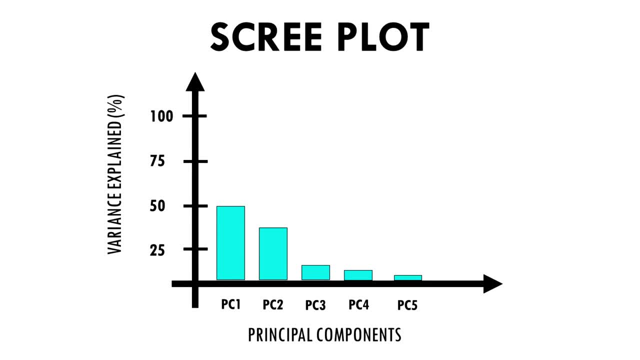 information is explained with each principal component. In this case, the first principal component explains 50% of the variance in our data set, So it's a very good way to analyze. This is amazing, by the way, with actual real-life datasets if you get close to 40%. 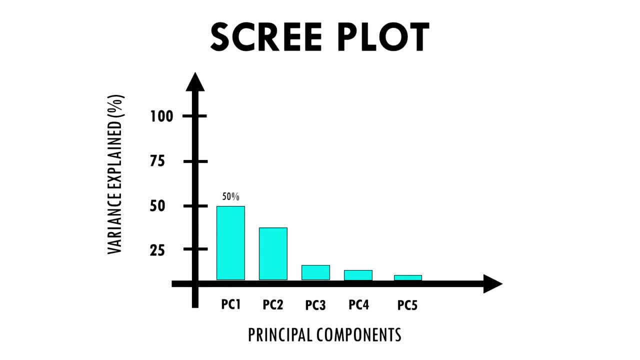 you might as well throw a party. Anyways, what this says is that 50% of the variation of a person's lifespan can be explained by principal component 1.. If you add principal component 2, that's another 35%, which makes 85%. Of course, it depends on your objectives. 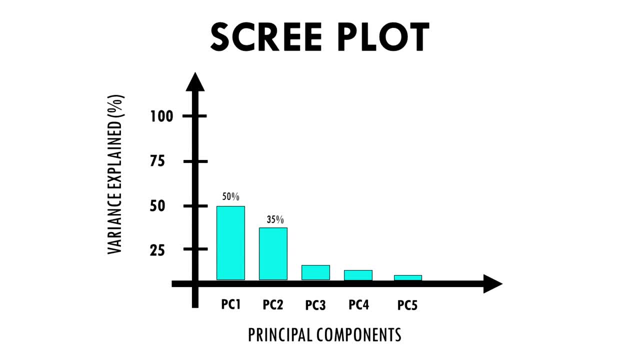 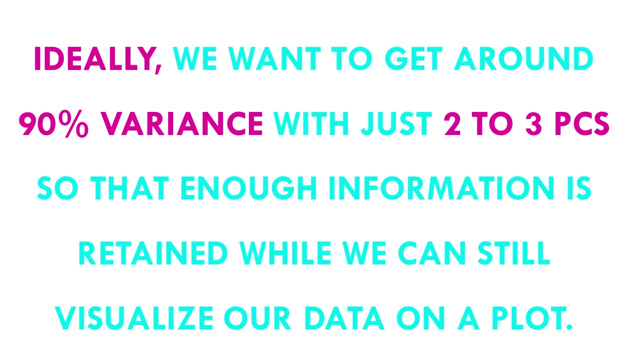 but explaining 85% of variance in life expectancy sounds quite nice to me. Ideally, we want to get around 90% variance with just 2-3 components, so that enough information is retained, while we can still visualize our data on a plot. Okay, but what is exactly principal component? 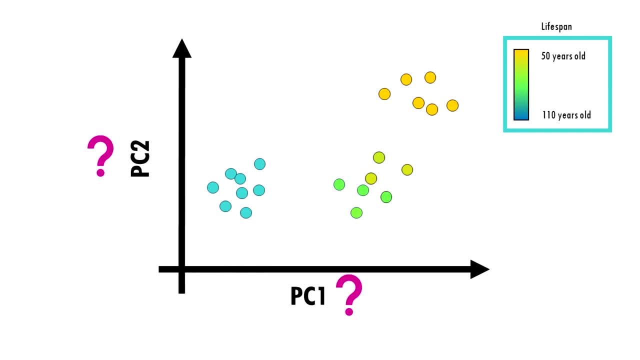 1?. What does it mean? As a biologist who's interpreting biological data, you're interested in knowing which variables or biological factors are responsible for the patterns you see among the observations or people. We would like to know which variables are influential and also how the variables 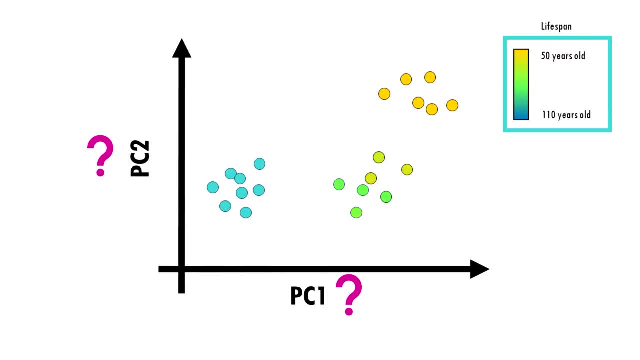 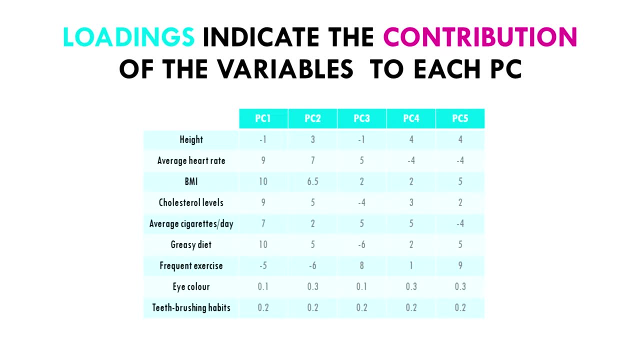 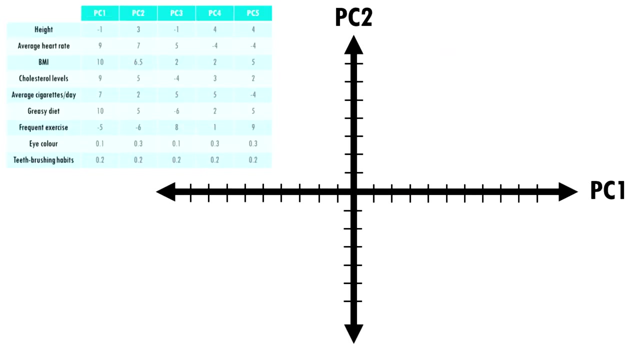 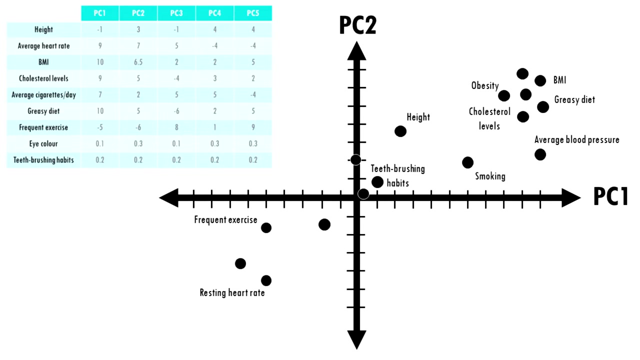 are correlated. This is given by the principal component loadings. Basically, each variable gets a loading or weight for each principal component, which tells you how much it contributes to that PC. We can also plot the loadings to see the relationship between our 200 variables. let's just plot some of them, for example for pc1: 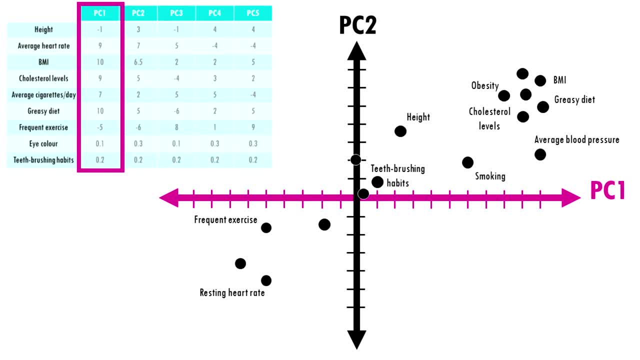 which again is the most important pc. we might expect to see variables like greasy diet, obesity, heart rate or frequent exercise to have really large weights, because they contribute a lot, and maybe variables like how many times you brush your teeth a day have a lower weight. so each of 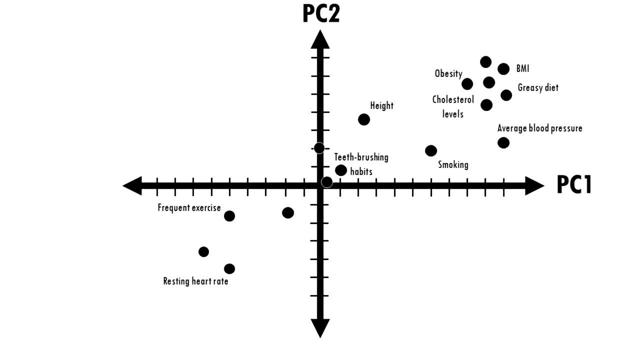 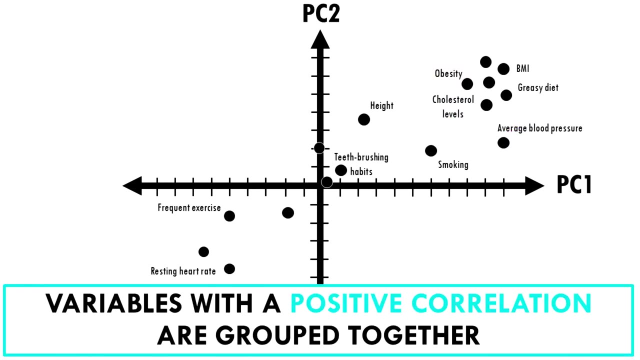 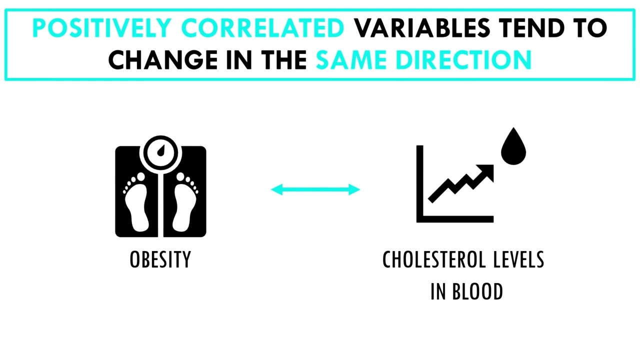 our 200 variables gets a loading score or weight for each principal component. you might have noticed that variables contributing similar information are grouped together. this is part of the magic of pca. variables that are positively correlated- for example, greasy diet, obesity- are grouped together. correlated just means that when the numerical variable of 1 increases or decreases, 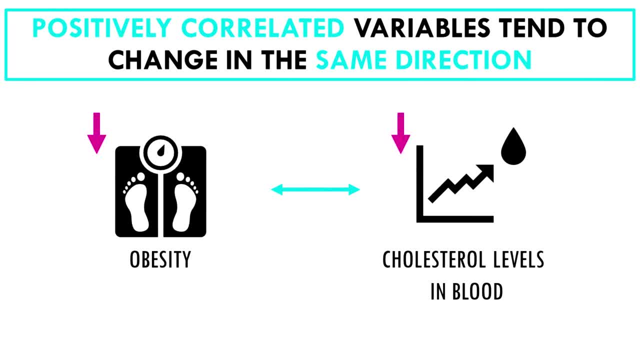 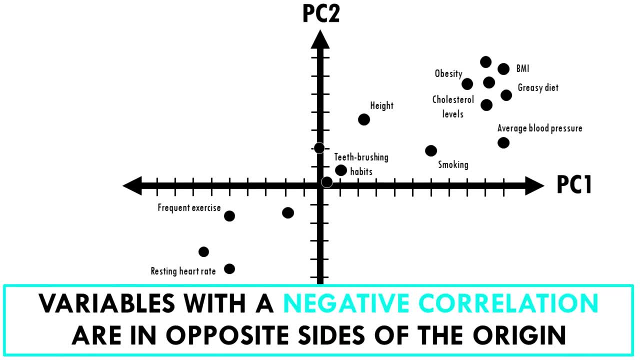 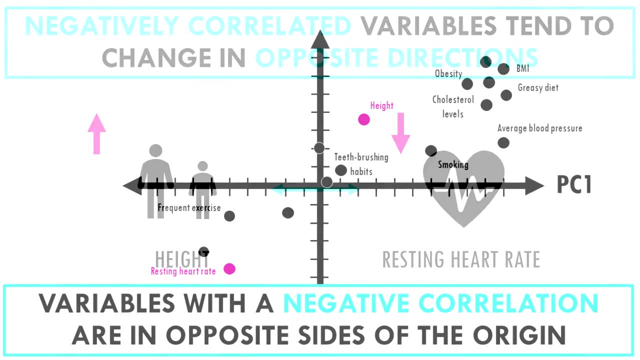 the numerical value of the other variable has a lot more value, a tendency to change in the same way. On the other hand, when variables are negatively or inversely correlated, they are positioned on opposite sides of the plot, origin in diagonally opposed quadrants. For example, your resting, heart rate and height are inversely correlated. 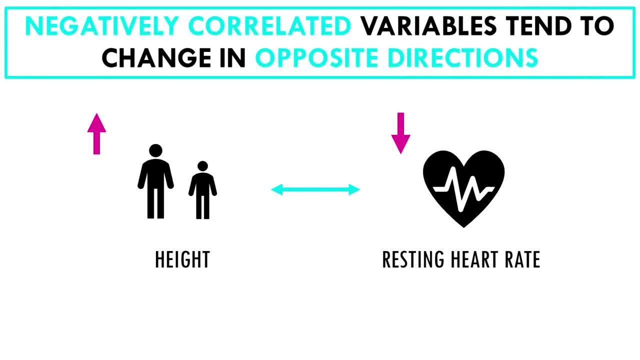 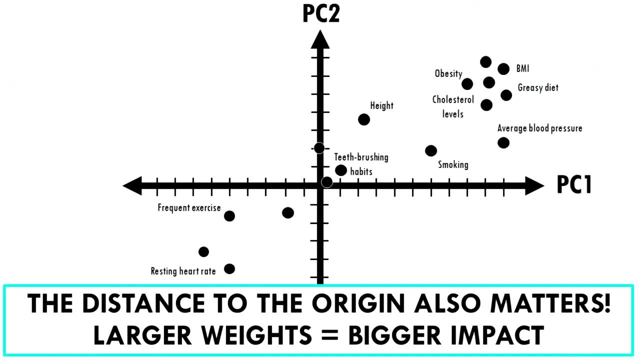 meaning that taller people tend to have lower resting rates compared to shorter people. Moreover, the distance to the origin also gives you information. The further away a variable is from the origin, the stronger the impact it has on the model. For example, here, obesity, blood pressure and average heart rate seem to be good variables to separate. 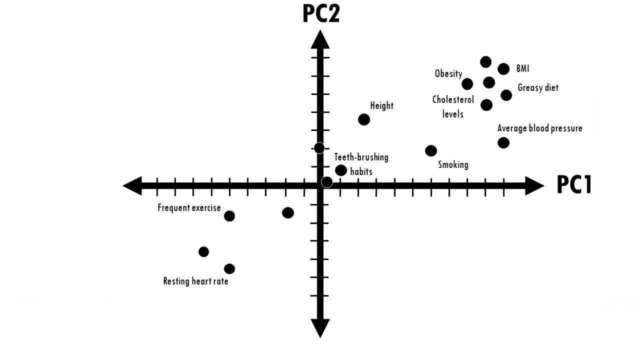 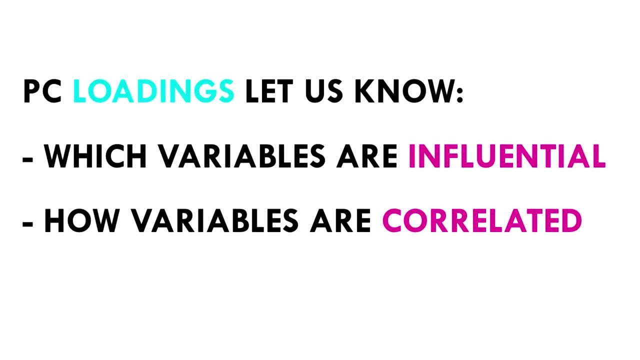 longer lifespans from shorter lifespans. So this loading plot is a great way of seeing the relationship between our 200 variables. at the same time, It lets you know that the relationship between our 200 variables and our 200 variables is not always the same. It lets you know what variables are influential and also how the 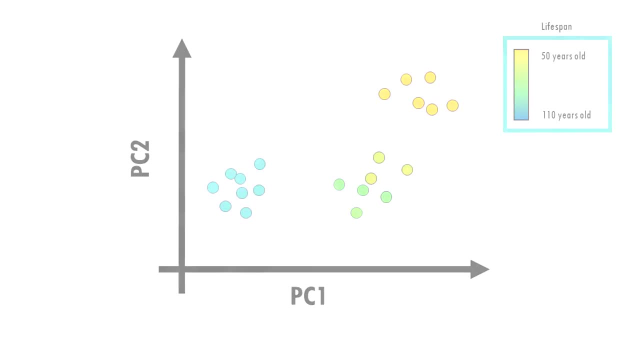 variables are correlated. Okay, so back to our PCA plot. How do we use this to draw conclusions from our dataset? Let's have a look at this other example. We have data from the gene expression profile of 50 different patients with lung cancer, And for each patient we measured the expression. 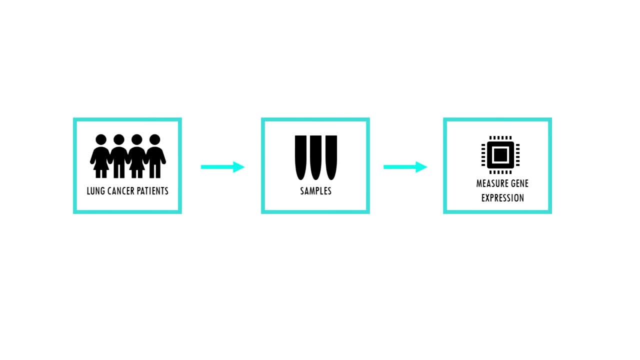 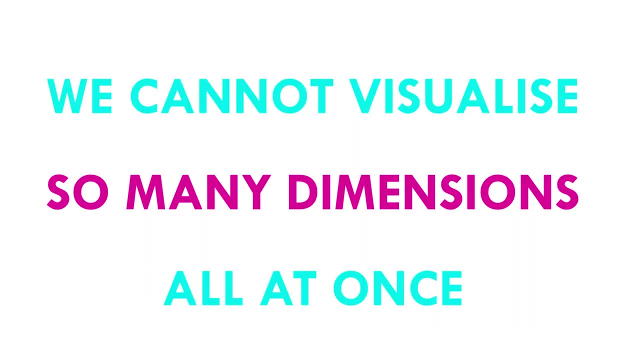 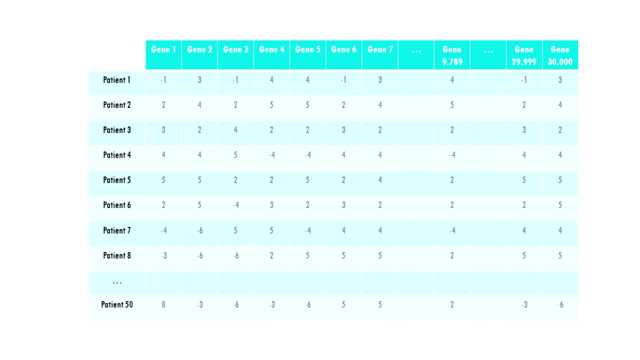 of 30,000 genes. We could plot the expression of genes individually across all patients, but we cannot visualize the expression of all genes across all patients all at once, Or can we? To get a general overview of our data, a good place to start is with PCA. 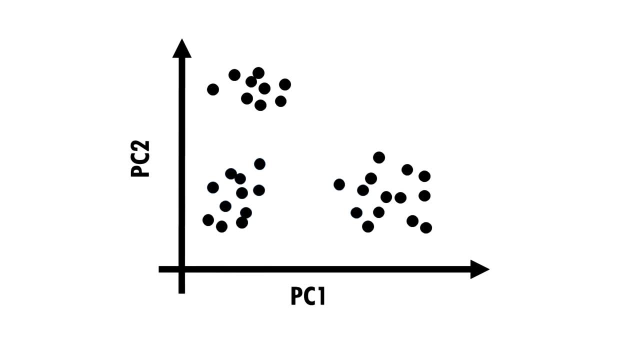 So this is our PCA. Each point is one of our patients. Patients with similar gene expression profiles are now clustered together. Just glancing at this plot, we can see that there are three clusters of patients. This means that overall, we have three distinct gene expression profiles, And this is very interesting because it 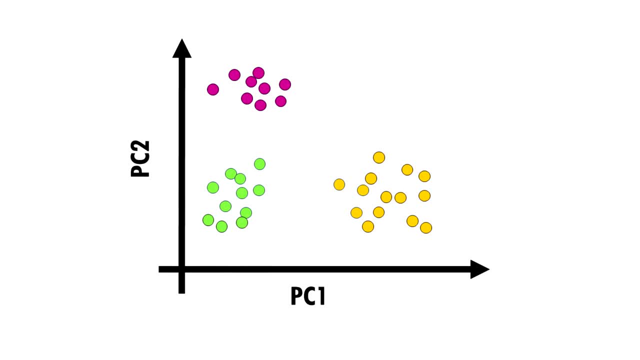 might mean that this group of patients will respond better to drug X and this other group of patients will respond better to radiotherapy. Now the orange and green clusters are different based on PC1. So the differences in gene expression profiles are probably due to genes that 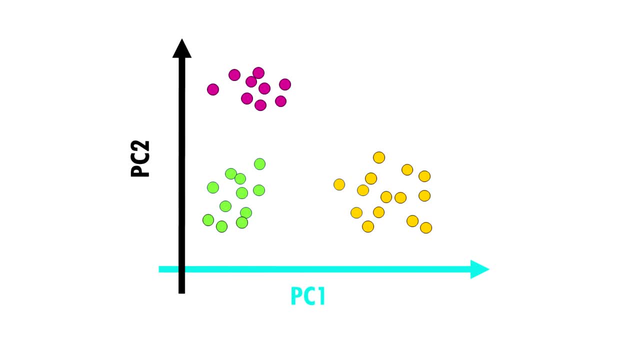 have heavy influences on PC1. Remember that the loadings tell us which genes have heavier weights on the principal component. The pink and green clusters are different based on principal component 2. So the genes that influence PC2 are more likely to be responsible for this. But remember, principal components are actually 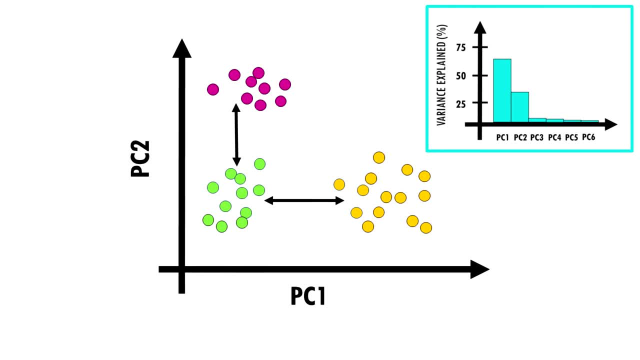 ranked by how much they describe the data, PC1 is more important than PC2.. So actually differences between clusters along PC1 axis are large, rather than the similar looking distances along PC2 axis. So here clusters green and orange are more different amongst each other than clusters green and pink. 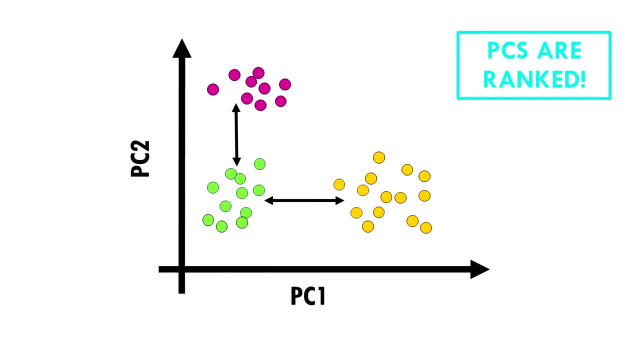 Wait, but are two principal components enough to represent all our 30,000 genes? Perhaps you remember how to check this? That's right, we need to take a look at the scree plot. In this case, the first two principal components cover most of the variation in our data set. 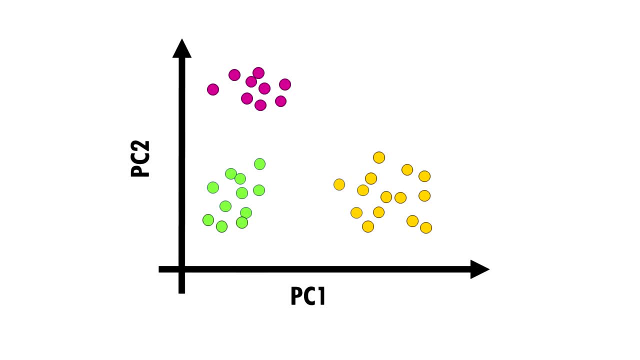 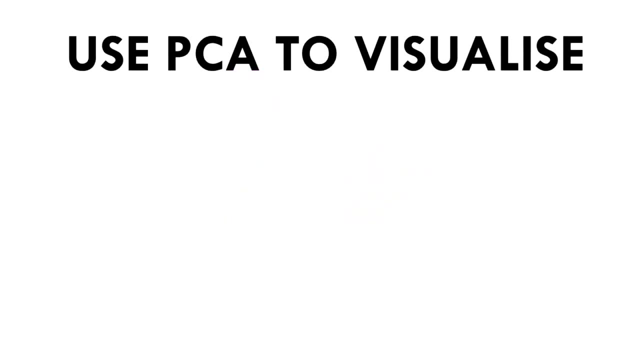 So they're good enough, And this is one of the first steps of analysis. As you can see, PCA is a great way of representing large data sets, to observe trends, jumps, clusters and outliers. From here we would of course trace back to find out which genes make the clusters different from. 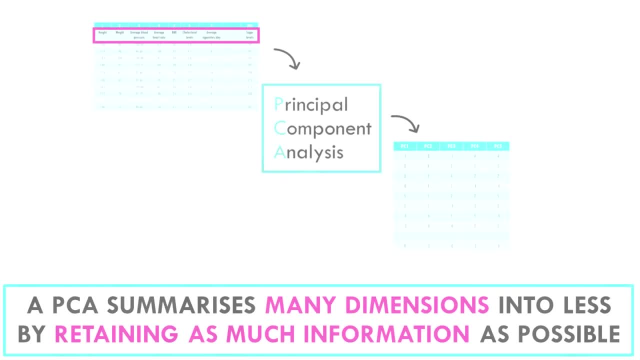 one another. So, to sum up, PCA is a great way of summarizing large data sets with many dimensions into less dimensions. PCA is a great way of summarizing large data sets with many dimensions into less dimensions, While retaining as much information as possible. It captures the essence of 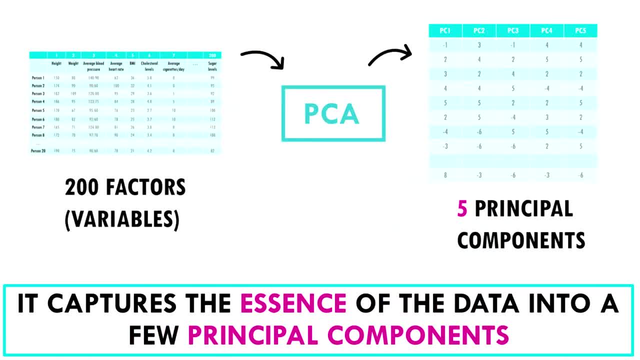 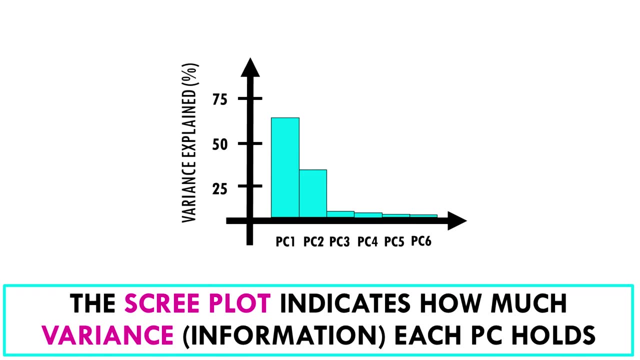 the data into a few principal components. Usually it's enough to keep just the first two or three principal components- if they explain enough percent of the data set. To check how much variance or information the first few principal components hold, you should look at a scree plot. How do we read a PCA Observations with similar overall profiles. 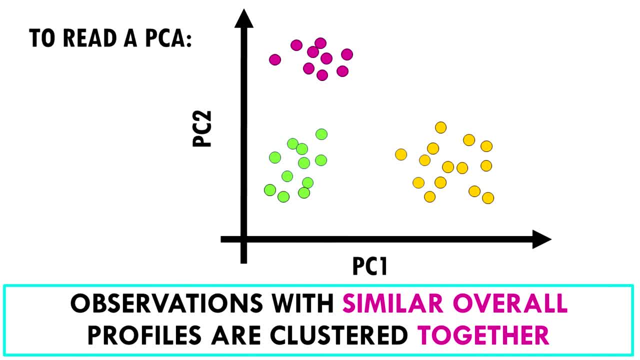 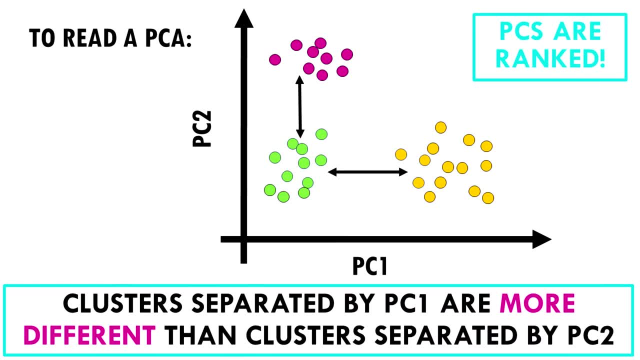 are clustered together. PC1 captures the most information from our data set, followed by PC2, and then PC3, and so on. This means that clusters separated along the x-axis are more different than clusters separated along the y-axis by a similar distance, If you're interested in understanding how PCA actually works, so 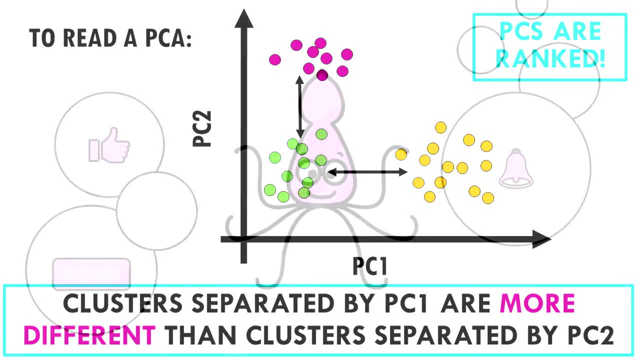 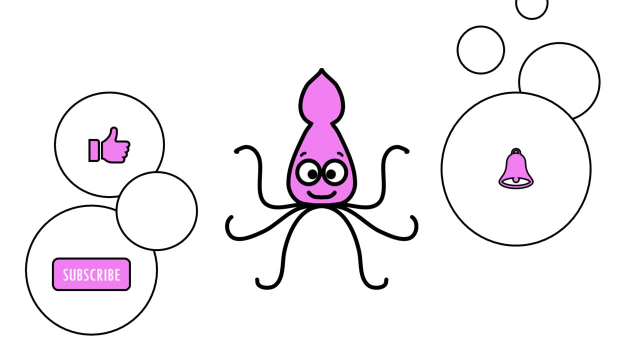 how it is able to understand and summarize the data. leave me a comment down below. I will try my best to explain it with zero math so you can get an idea of how it does it. If you liked this video, let me know, and if you don't.